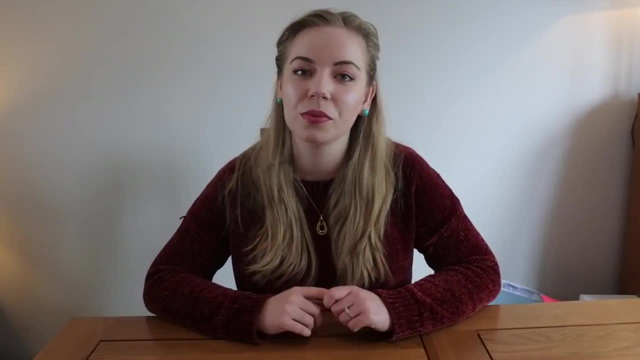 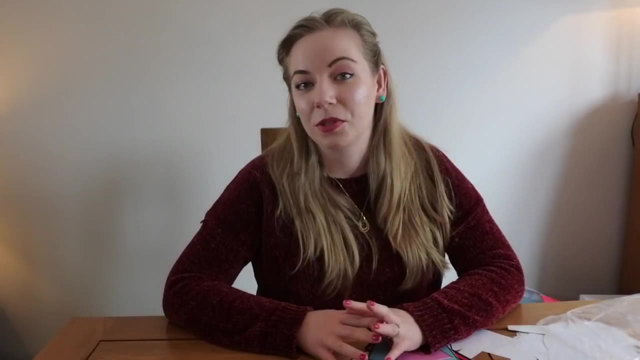 other ideas that you can do if you're trying to think of something you can do with your children during the summer holidays, for example, or just something you can do as a little bit extra at home. Now, obviously, children need the opportunity to see numbers. 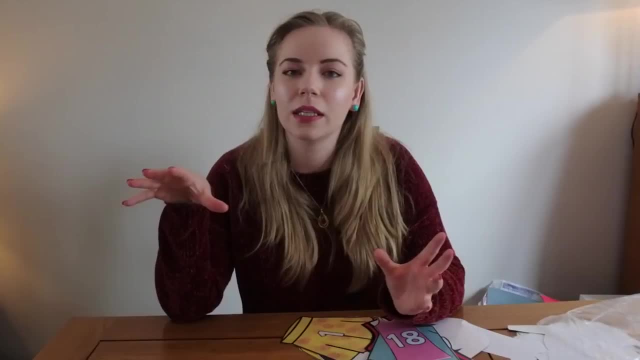 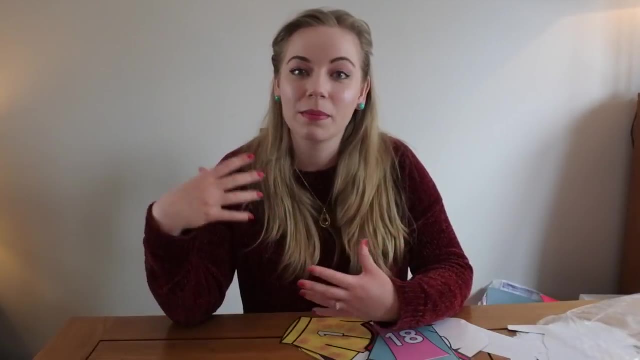 so it would be great if you could have some kind of wall chart. They're really easy to make or you can buy them really cheaply from Amazon or places like WH Smith. This video is not sponsored And it's great because then they just get to see them every day At the age children are in reception. 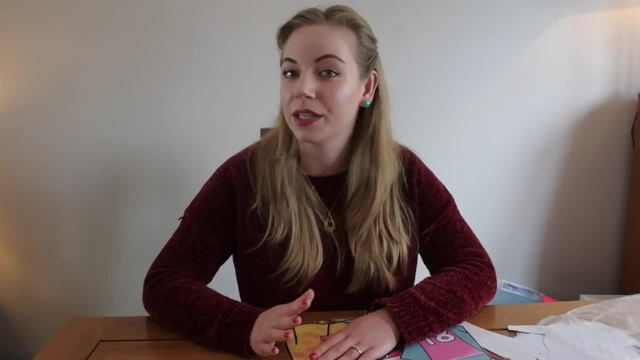 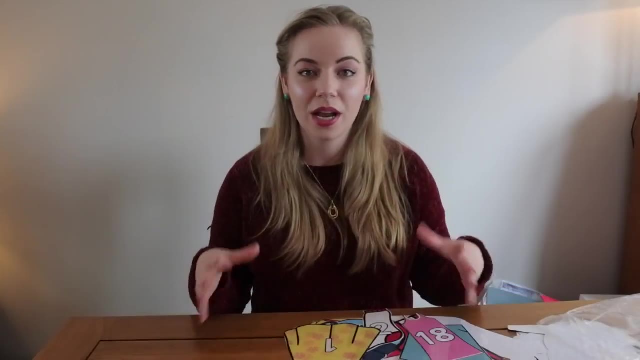 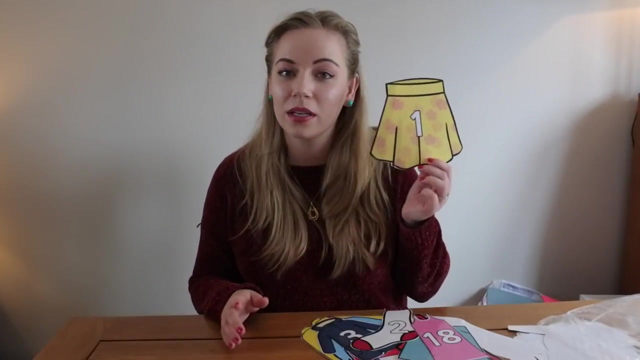 they learn so much through play, so it's brilliant if you can fit numerals into their regular play. One thing I really love to do is to put a washing line up. You can have a water tray or you can just have a bucket of water outside and you can print these. You can either 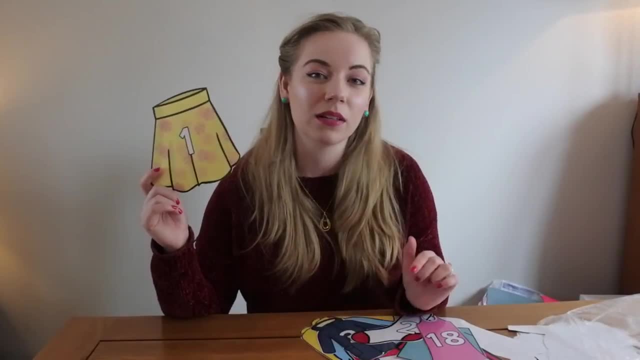 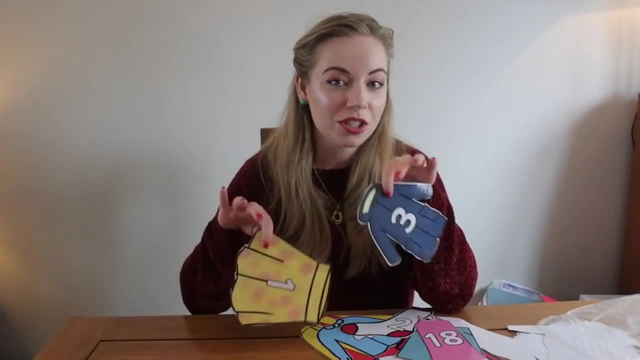 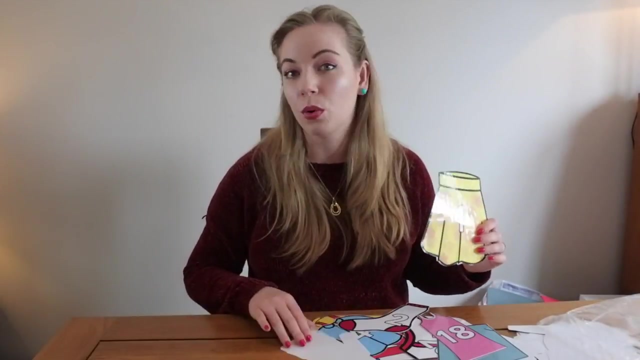 make them or you can print them from different websites- I'll link some down below- And they are clothes that you can laminate and then children can pretend to wash them in soapy water and then hang them up on the washing line. This is really good for recognising the numerals, but also for 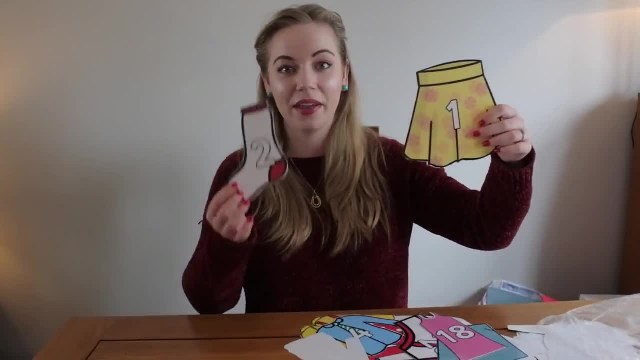 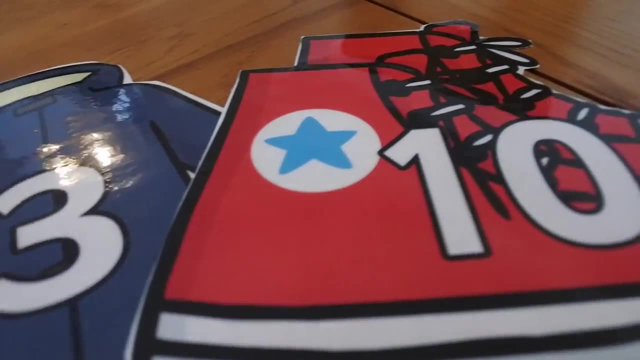 using them. So they put a number one up on the washing line and then they can peg up the number two on a washing line. Children really love this idea because they see Mummy and Daddy putting clothes on the washing line all the time and they love to play being grown up. So these are 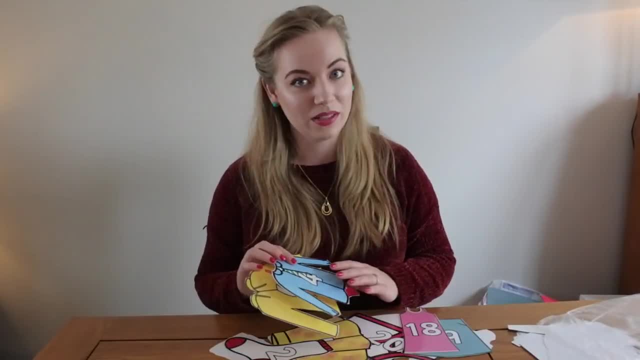 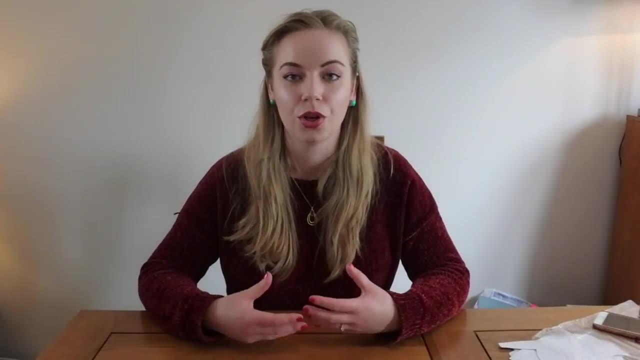 fantastic. I've used them in my classroom every single year and they are always a winner with the children. You can also do some fantastic sensory activities to do with recognising numerals. So you can make feely numbers which are just: you just print out numbers and then you can print out numbers. 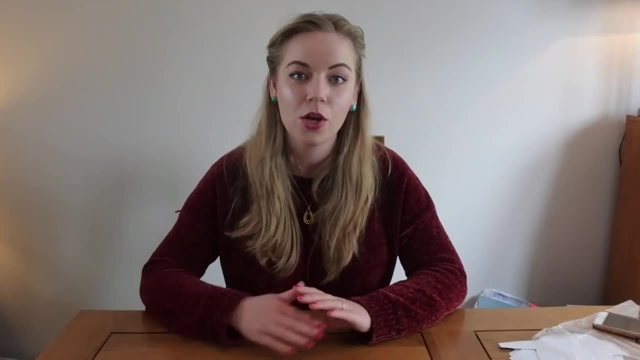 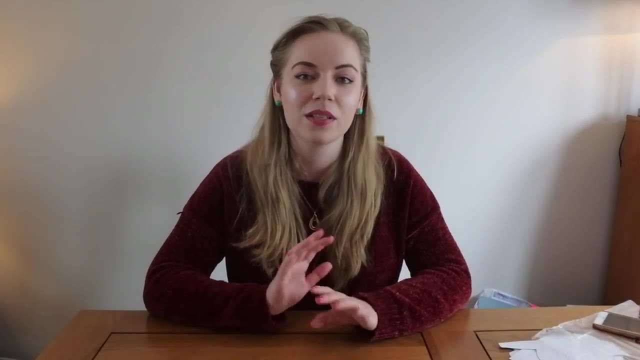 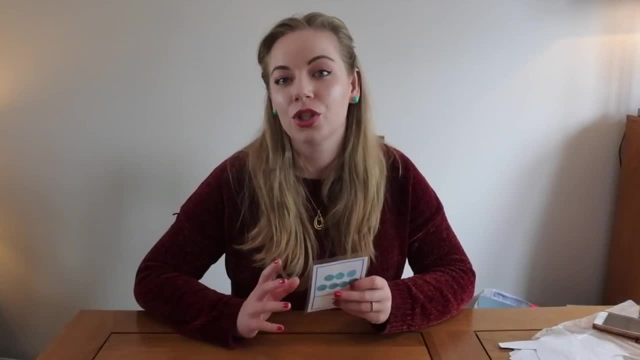 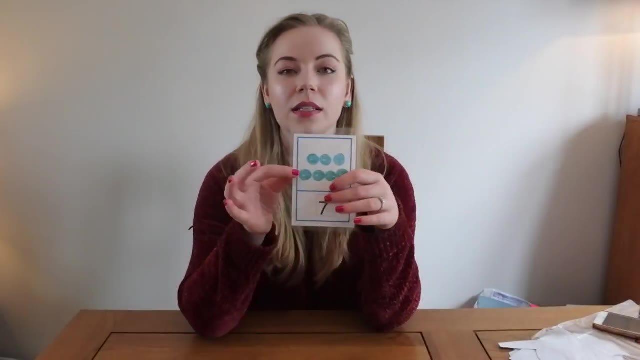 to help your child recognise their numerals. You can then move on to matching numerals to quantities. So, for example, in my classroom I used to have these little gems- Hopefully you can see those. They were blue, lots of different colours, and I would put them out in. 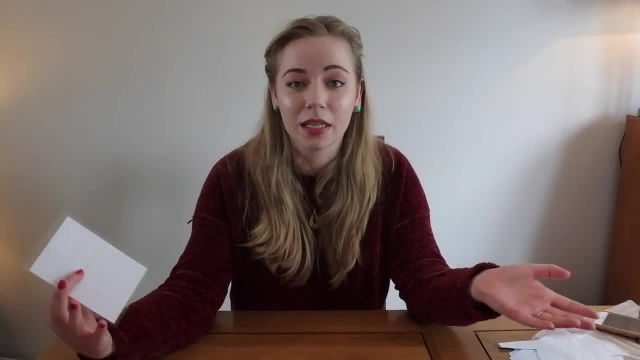 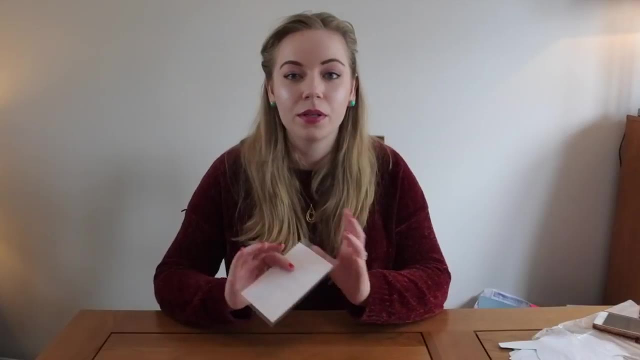 the play area. So, for example, we might have a pirate table out with all of the ocean toys and the boats and the pirates and the fish and all of that, And I'd put some gems, scatter them around the table and then I'd put these cards around the table so the children knew that there were. 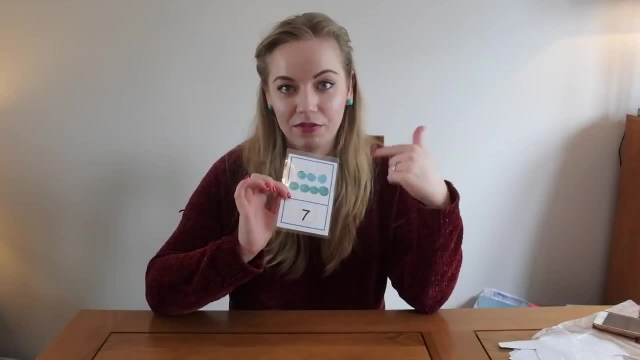 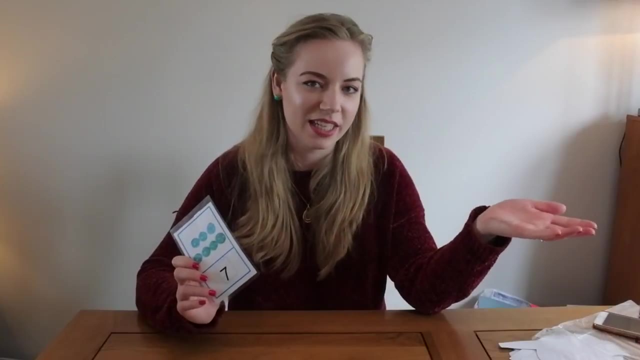 seven of these blue gems And once they found the seven, they would bring this card and the seven gems to me for a reward, usually a sticker. So obviously at home you don't need to print, print these out and laminate them, I just have this because I had it in my classroom. 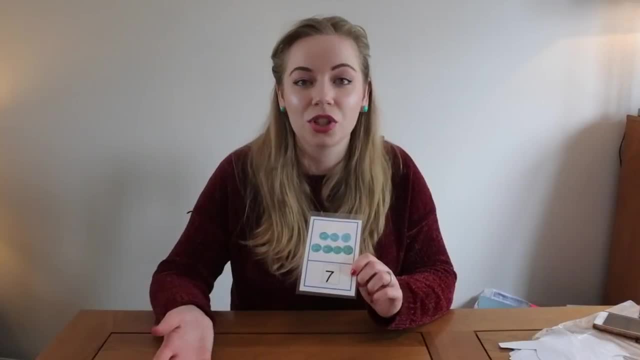 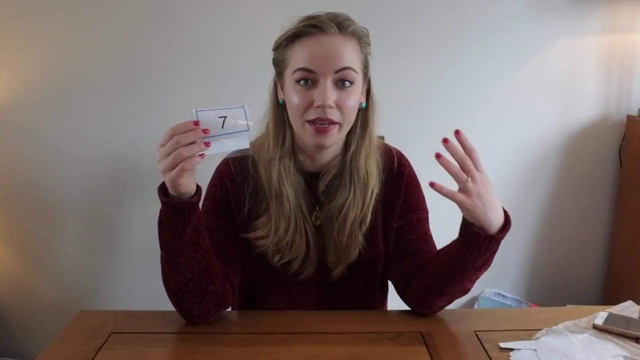 But you could have the numerals around the table and ask your child to find this many red pieces of Lego. So they obviously need to know that that's a seven and then they can find seven pieces of Lego. So that's using their counting And then they're matching the quantity. 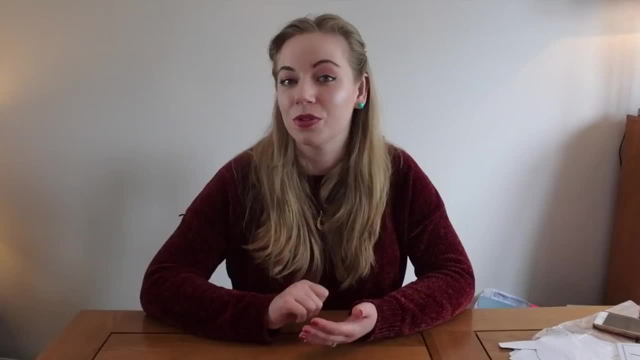 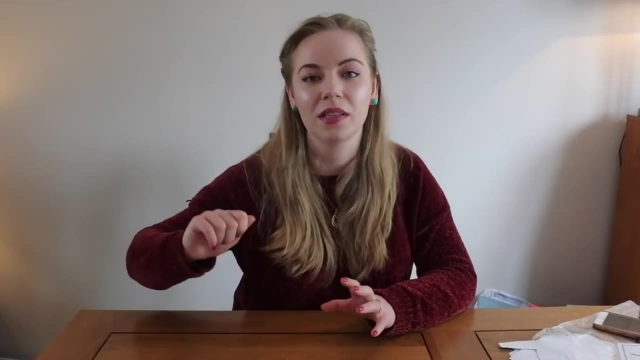 to the numeral. Another fun idea is to just write numerals on post-it notes and stick them around the house So you can go for a number hunt and your child can go and look for them, find the post-it note and tell you what the number is. So those are just some really quick. 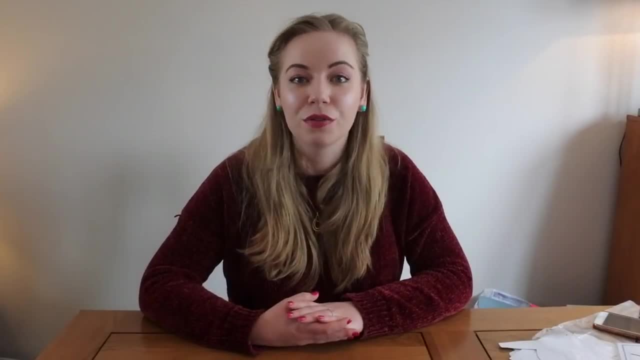 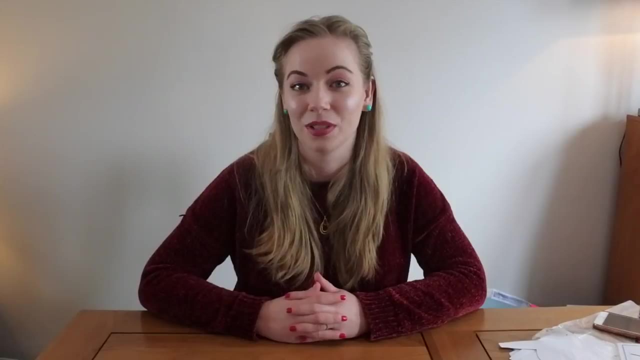 and easy ways you can help your child to recognise numerals at home. Of course, with all learning, repetition is key. Don't worry if it takes them a while to work out what each numeral is, or if one day they know what a five is and the next day they've forgotten. It just takes a lot. 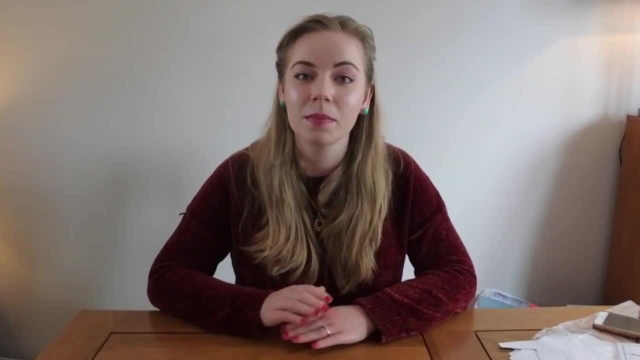 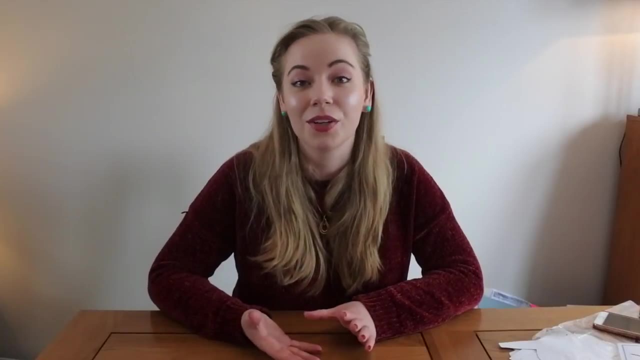 of practice. I hope you found this video helpful. If you did give it a thumbs up, Please do let me know in the comments below if you've got any tips and tricks for helping children to recognise numerals at home. I love to hear your ideas And also, obviously, it's great for parents. 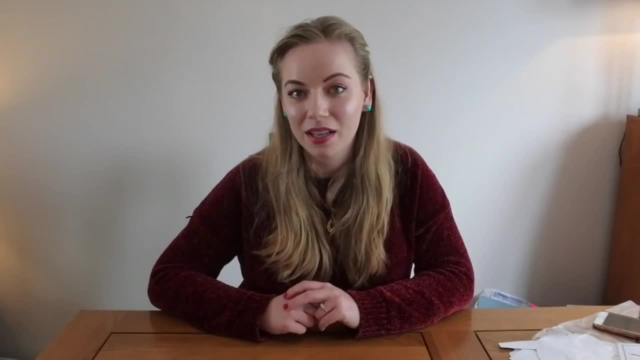 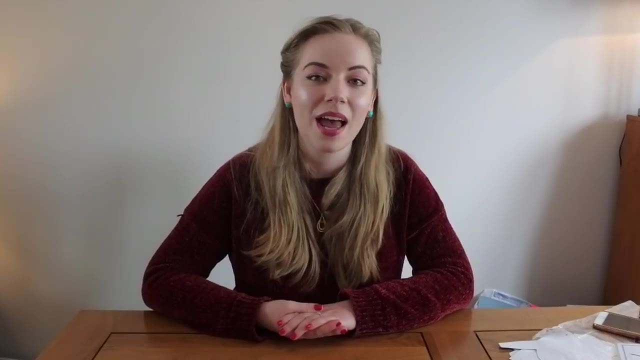 to be sharing with each other in the comments too. If you'd like to see more videos like this, don't forget to hit that subscribe button, And if you're already subscribed, you can click on the bell icon so you get a notification every time I post a new video. 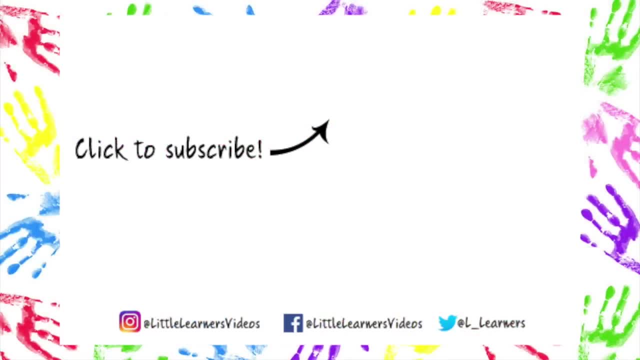 Thank you so much for watching and I will see you next time. Bye for now.